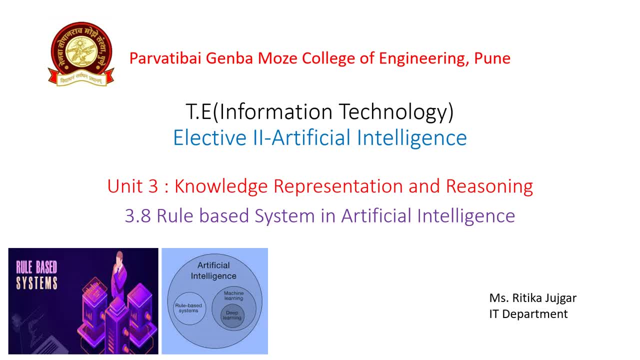 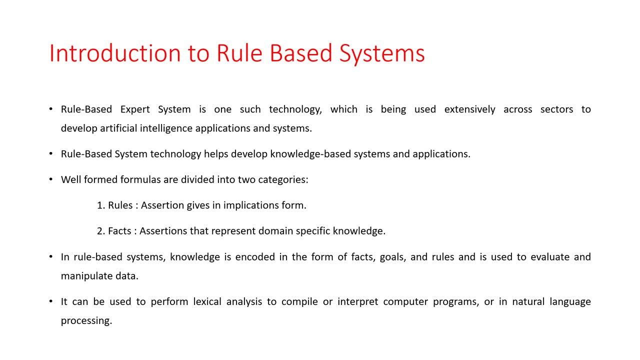 So here in this video we are going to discuss about this point. that is, the Rule Based System. So let us discuss here. The first thing is: So in the past few years the technology has experienced a drastic change, So in the field of Computer Science or in the field of Artificial Intelligence, 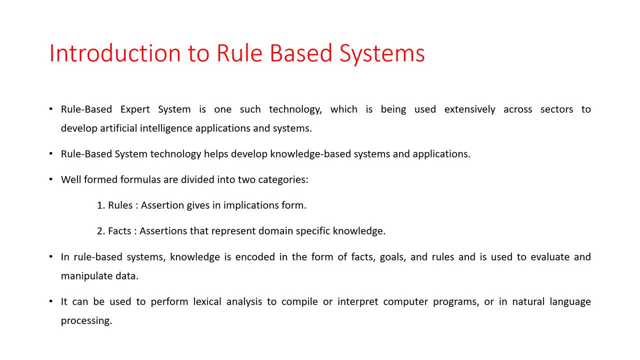 there are new, more advanced researchers and inventions have given way that machine delivers the excellence and help us to emit the human knowledge. So these new inventions are result of numerous technology that works behind the scene and it enables them to deliver the service that are a part of our humans. 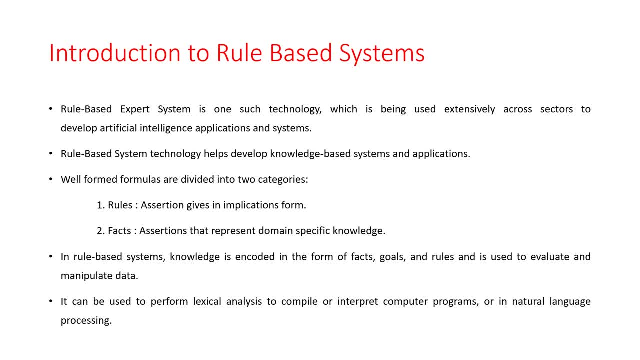 So the Rule Based System is one such technology which is being used extensively across the sectors to develop the Artificial Intelligence applications and system. So therefore, today we will explore the concept of Rule Based System, that is, RPS, and try to understand the roles in the research and the development perspective. 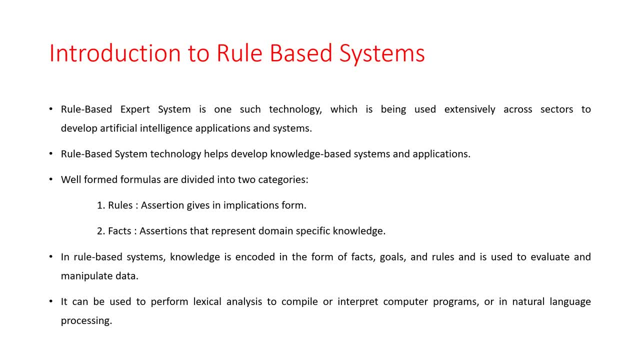 So what are the Rule Based Systems? So in the present, in the heart of automated processes, the Rule Based System technology helps to develop the knowledge based system and the applications. It helps to develop the knowledge based system and the applications, So that is, the intelligent programs and the software capable of providing the special 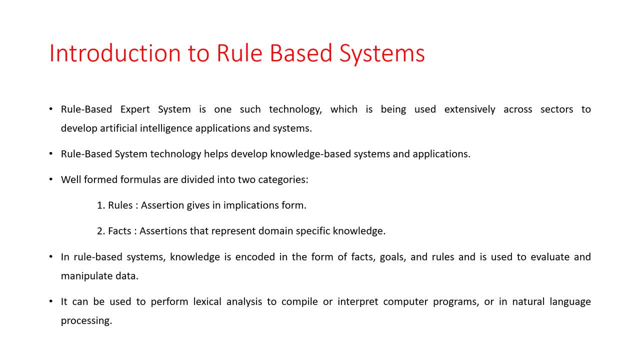 specialized problem solving expertise in a specific subject by utilizing the domain specific knowledge. So, in this Rule Based System, knowledge is encoded, is in the form of rules and facts, Rules and facts, and also in the form of goals, So and it is used to evaluate and manipulate the particular data. 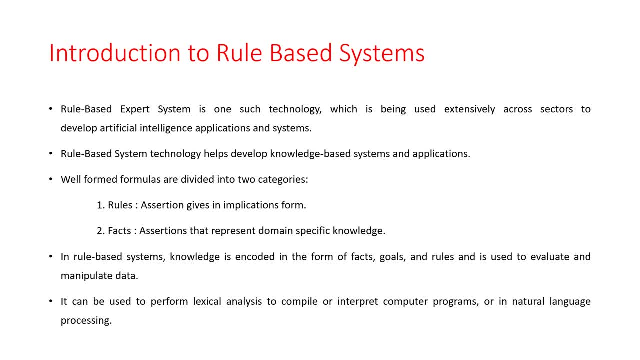 So these are, in short, in the Computer Science, the system that uses the rules to perform the variety of tasks like diagnosis to solve a problem, then interpretations, or to determine the course of actions in the particular situations. So these are applied to the system involving the human crafted, human crafted rule nodes. 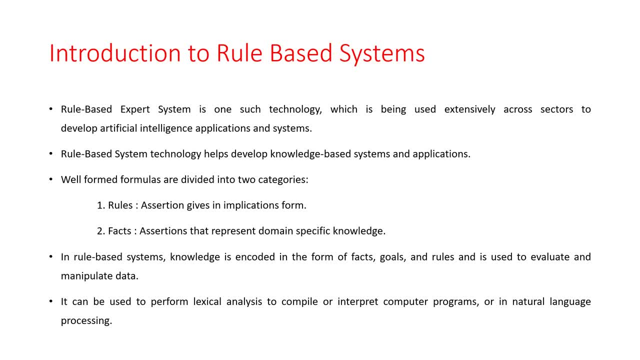 and it can be used to perform the lexical analysis, to compile or interpret the computer programs or, in a natural language, processing. So in the Rule Based System the well formed formulas are divided into the two categories Rules and Facts. So all these Rule Based Systems are used. are all these Rule Based System? Rule Based System. 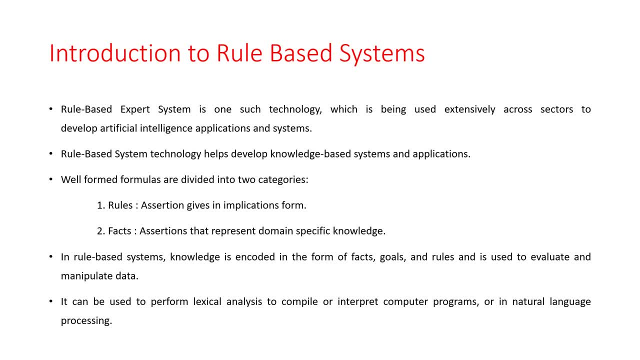 knowledge is encoded by using the Rules and Facts and Goals. Okay, So in previous lectures we already discussed about what is mean by Rules and Facts, which is in the form of a well formed formulas like Proposition Logic and Predicate Logic. Okay, 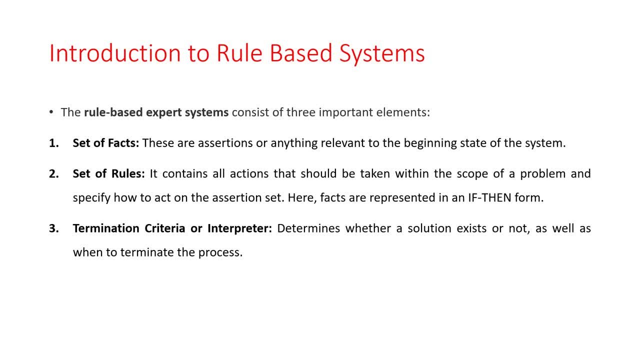 So the Rule Based System expert consists of the three important elements: First the set of facts, then set of rules and third thing is the termination criteria or the interpreter. So in the set of facts these are the assertion or anything relevant to the beginning state. 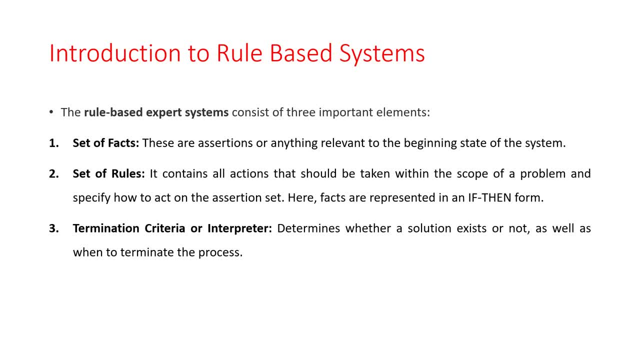 of the system. Okay, So in the set of rules we have, it contains all the actions that should be taken within the scope of a problem and specify how to act on the assertion set. So here the facts are represented in the form of if-then form. 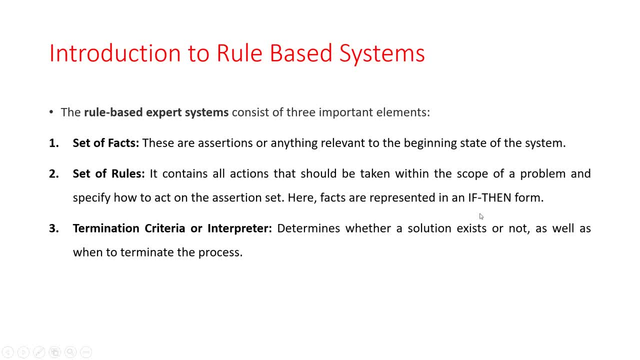 Okay, So this is the set of rules. If the particular condition is successful, then we have to perform this particular task. Okay, So there are different set of rules. And the third thing is the termination criteria, or the interpreter, So to determine whether the solution exists or not, as well as when to terminate the process. 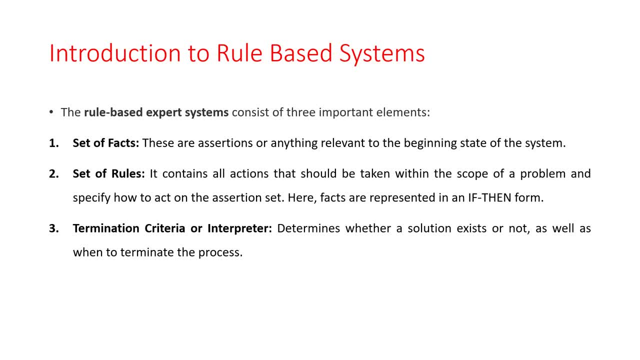 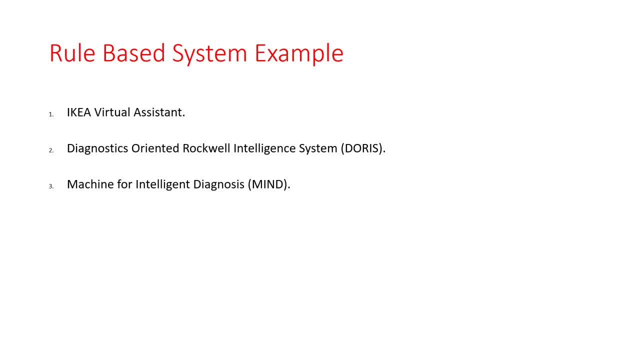 Okay, When to terminate the process? Okay, So this is a part of a termination criteria, or the interpreter. So next point is a Rule Based System examples. So in the domain specific expert system that uses the rules to make the deductions or the 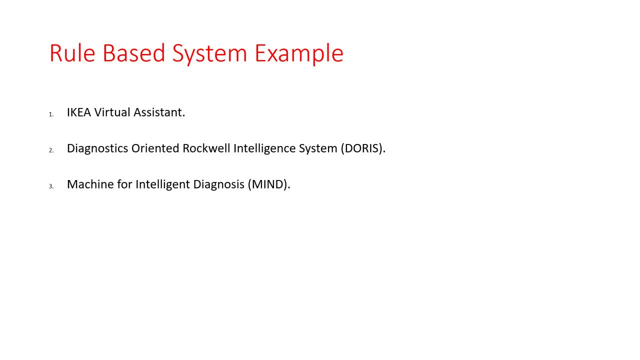 narrow down choices is one of the rules. This is one of the most popular as well as classical example of the rule based system. So in the recent advancement in the technology that has given a way to development of modern machines and the systems like IKEA virtual assistant, then diagnosis oriented Rockwell. 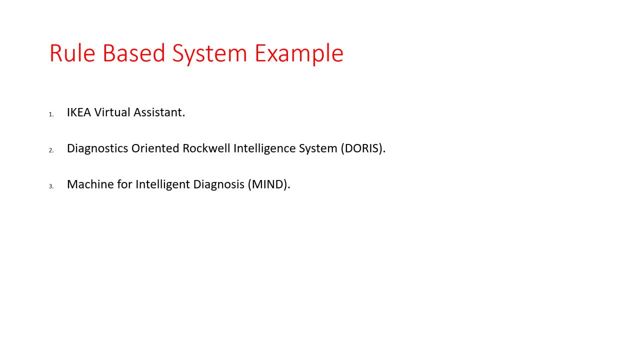 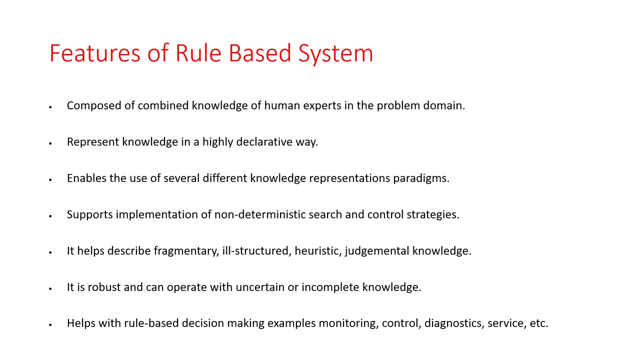 intelligent system, that is DORIS, and the machine for the intelligent diagnosis, that is MIND. Okay, So these are the. So these are the advanced, recent advanced rule based system examples. The next point is the features of rule based system. 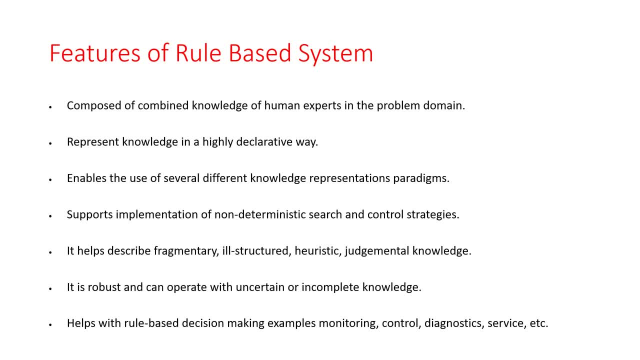 So rule based system is widely used in the artificial intelligence and it is not just only responsible for modeling the intelligent behavior in a machine and building the expert system And that outperform the human expert, But it also helps to compose the machine Okay. 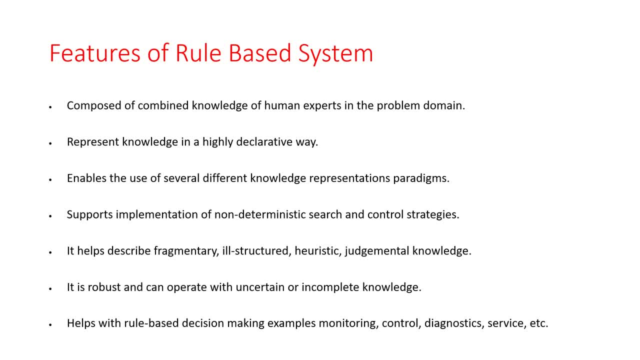 To compose of combining the knowledge of human experts in the problem domain. Then represent the knowledge in the highly declarative way. Okay, Then enables the use of several different knowledge representation paradigms. Then support the implementation of non deterministic search and control strategies. 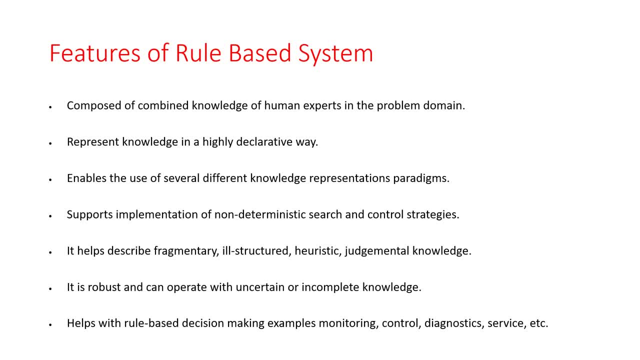 And it also helps to describe the also describe the fragmentary structure, heuristic judgmental knowledge. It is just robust And can operate with the uncertain or incomplete knowledge And it also helps with the rule based decision making. examples: monitoring, control, diagnostics. 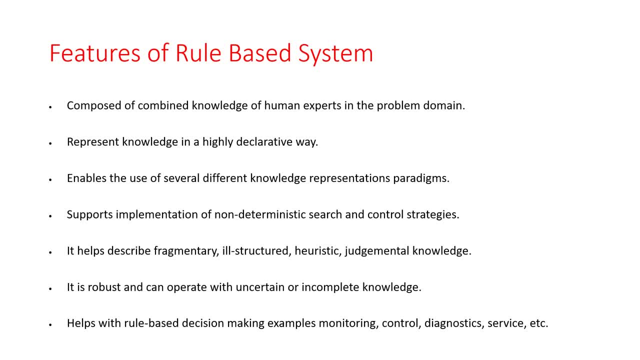 and services, etc. Okay, So these are the features of rule based system, rather than providing the intelligent behavior in machine and building the expert system to the human expert. Okay, Then the next thing is the construction of rule based system. Okay, 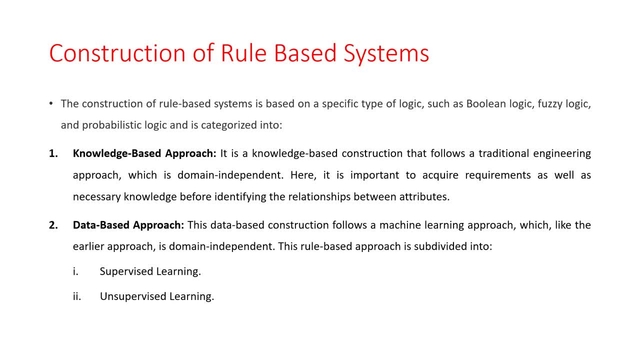 So before we move on the discussion the types of rule based system, we need to understand its construction. Okay, So in the next video we are going to discussing about the types of rule based system. So there are two types of rule based system, that is, the forward chaining and backward. 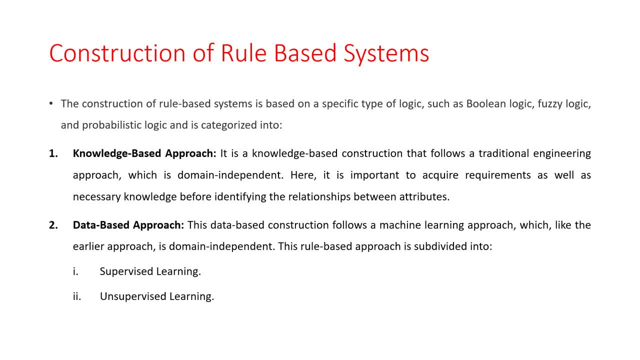 chaining. So before starting the types of rule based system, first we have to learn about the construction of rule based system. Okay, So the construction of rule based system. So the construction of rule based system is how the system evaluates the information. 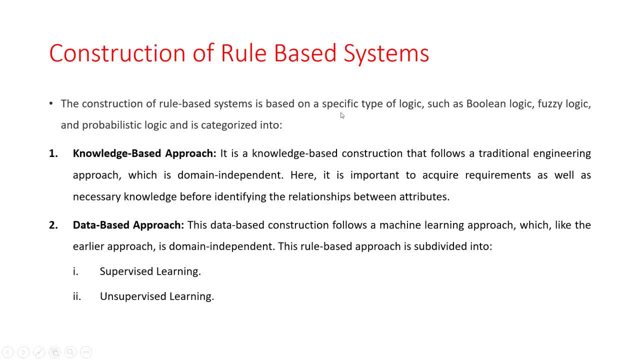 So the construction of rule based system is based on the specific type of logic, Based on the specific type of logic, such as Boolean logic, fuzzy logic and probabilistic logic. Okay, So it can be characterized into the two parts: First is a knowledge based approach and second one is a data based approach. 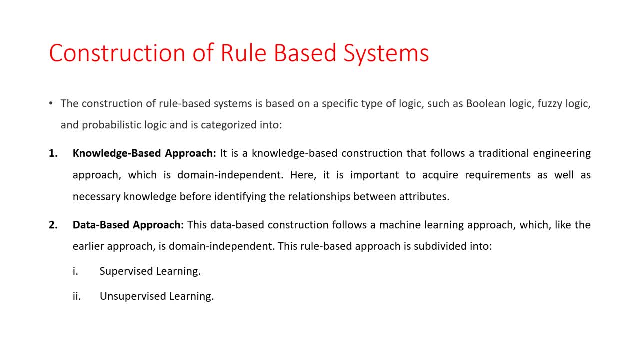 So in the knowledge based approach, It is a knowledge-based construction that follows the traditional engineering approach, which is a domain independent, which is a domain independent. So it is important to acquire the requirements as well as necessary knowledge before identifying the relationship between the attributes, relationship between the attributes. and the second thing is the data-based approach. 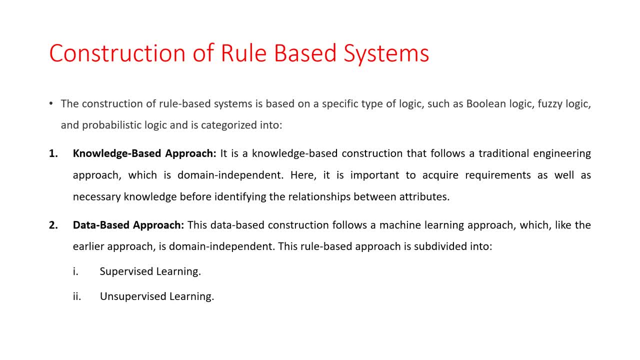 So this data-based approach or construction follows the machine learning approach, which, like the earlier approach and it is a domain independent. So this rule-based approach is subdivided into the supervised learning and the unsupervised learning. So, whatever is the knowledge-based approach, how we will study the rule-based system based on the knowledge. 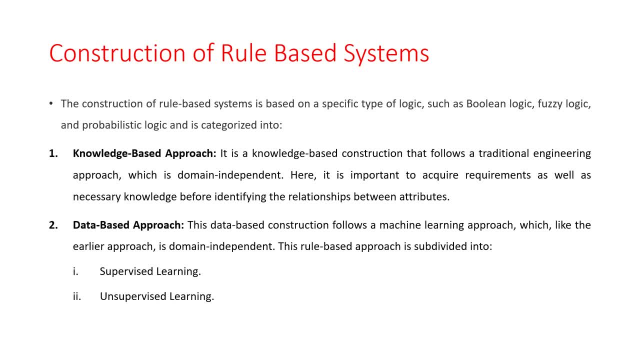 So, based on the knowledge, what we will do on the previous knowledge, we will improve our system. So this is the knowledge-based approach. So the data-based approach means that where we have two data given, we will work on that data and in that way we will provide the learning technique to our machine. 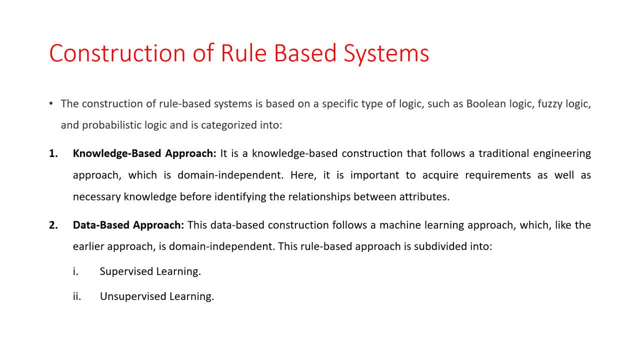 That is supervised learning or unsupervised learning. Supervised learning works on the label data. Already we have some label data. it will work on it and will give us a solution, will give us some conclusion. And unsupervised data: The unsupervised learning technique works on the un-label data. 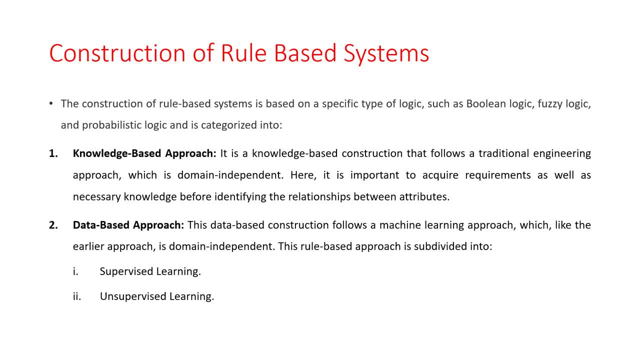 Because we don't have any label data given. So what we will do with that? we will solve the unsupervised learning technique, For example. the example of supervised learning is that we have a small child. He doesn't know any ABCD at the initial time. 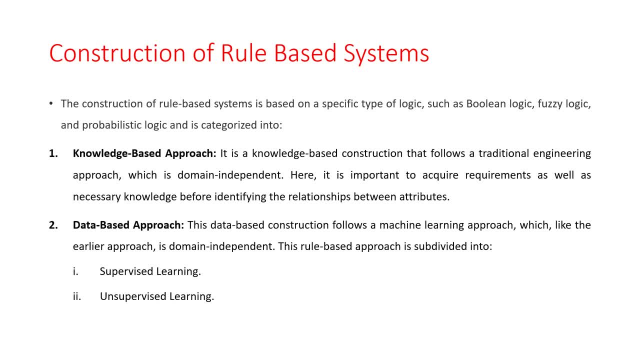 So under supervision, or under teacher or under parent, what he does is that he analyzes and learns new things. So under the supervision, whatever work we will do, whatever machine will learn will be supervised. learning Meaning we will have some label data, we will work on it and what the machine will do is learn. 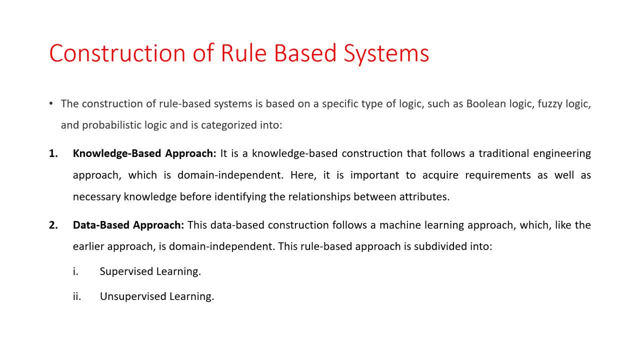 Unsupervised learning means what? It does not have any label data given It will learn new techniques through unlabeled data. Okay, As an example of supervised learning can be another. What we have to do is that we have multiple animals: images of cats, dogs and other animals. 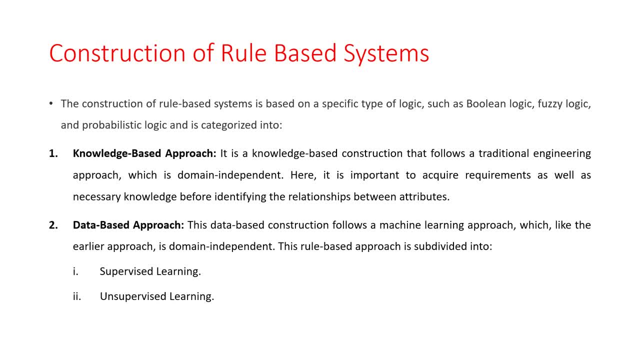 We have a label data to find out the images of cats. We will match the label data of cats with the given data of animals. We have a data of thousand number of animals. We will compare the label data with the image of cats. Through the label data, we can divide the images of cats from the images of animals. 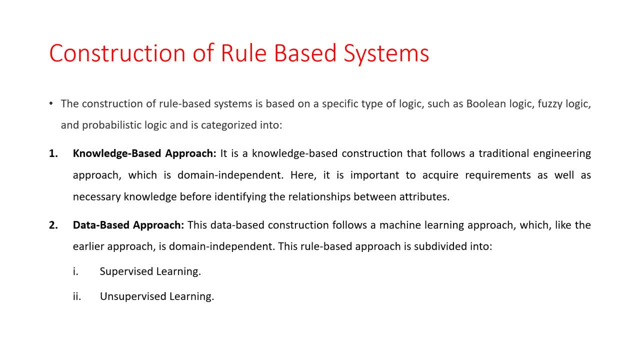 We can classify the images and make a group. This is a supervised learning which is called as a database approach. Another database approach is unsupervised learning technique. We don't have any label data. We have images of multiple animals. We have to group the images of multiple animals. 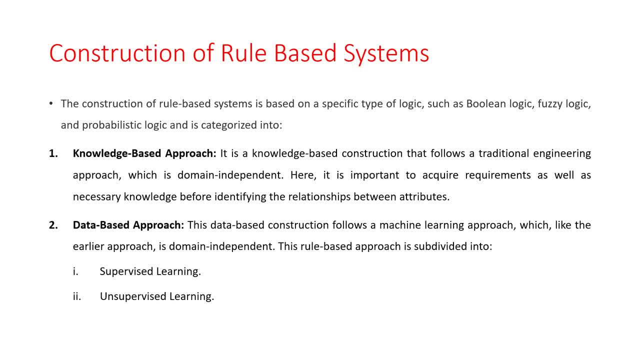 If we have a data of thousand number of animals, we have to make a group of cat images and dog images. from the data of thousand number of animals We have to group the images of other animals. The label will not work on the data. 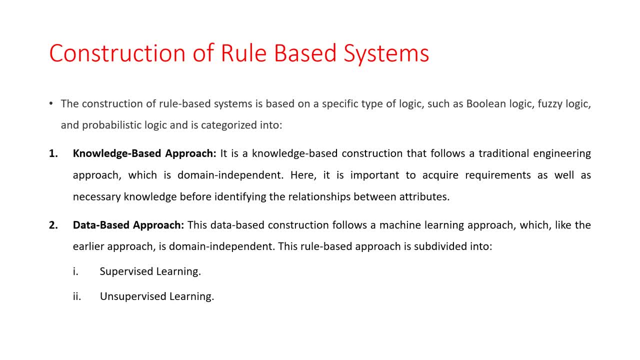 It will work on the features. We will match the data of some animals with the data of other animals. If the features of the first cat image matches the data of the second cat image, it will look similar. Without label data, we can group the data of the number of animals. 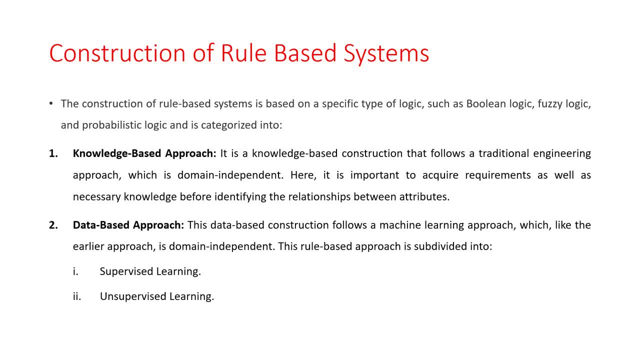 This is an unsupervised learning technique. Both these techniques are database approach. In the rule-based system, we are constructing the logic and rules. We are understanding and conferring logic and rules based on knowledge and based on data. The next thing is the advantages of the Rule-Based system. 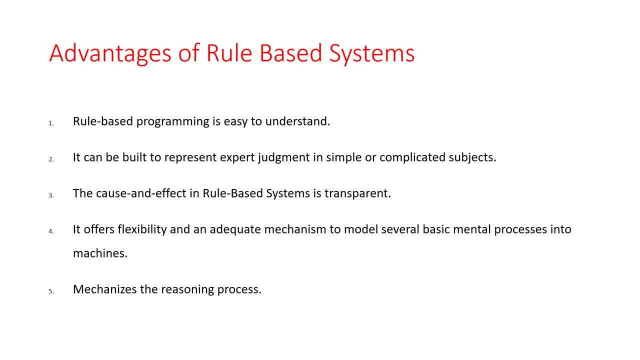 Which are the advantages? The rule based system is one of the core technologies which makes the machine hour master able to perform the rules-based learning. Rule based learning offer a range of advantages. like rule-based system, rule-based programming is easy to understand. it can be built to represent the expert judgment in the simple or complicated 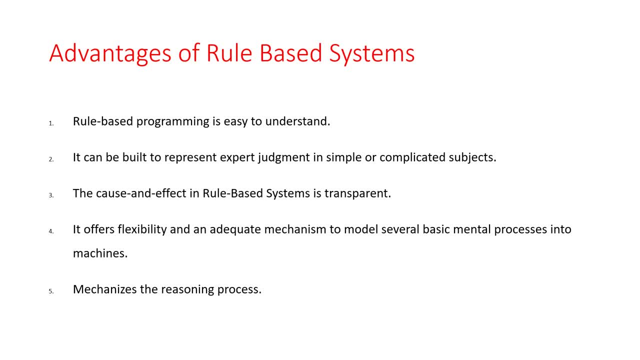 subject. it has a cause and effect in rule-based system. it is transparent, it offers the flexibility and adapts the mechanism to model the several basic mental processes into the machine. and last thing is a mechanize, the reasoning process. okay, so these are the advantages of the rule-based 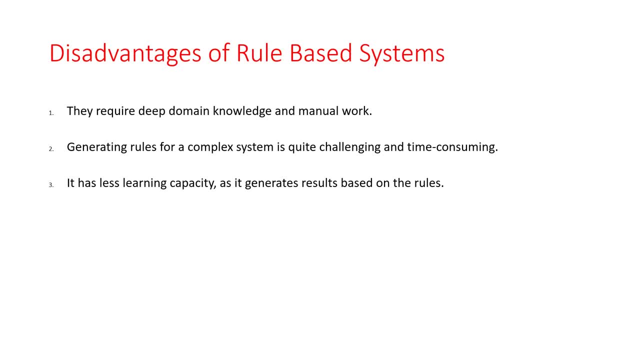 system and what are the disadvantages of this rule-based system so truly exponentially? when we see here the rule-based system, have the certain problems associated with them, such as: they require the deep domain knowledge and manual work. require the deep domain knowledge and the manual work. then generating the rules for a complex system is a quite challenging. 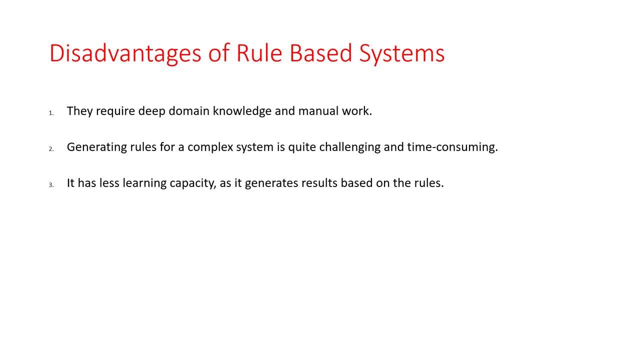 and time-consuming, because each and every time, for each and every system, we have to generate the rule. okay, so, because of this generating the rules, it becomes a complex system and it is a quite challenging and time-consuming process. and the last point is it has a less. 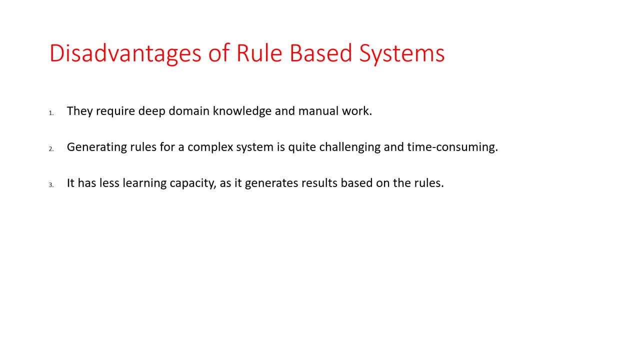 learning capacity as it generates the results based on the rule. okay, so based on the rule, here we have a less learning capacity because whatever we have learned in the last few years, we have generated the results based on the rule generally. and the next thing is the: 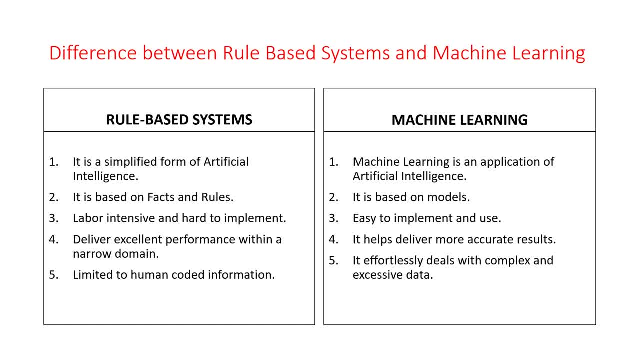 difference between rule-based system and machine learning. so what is the difference here? in the rule-based system we have, it is a simplified form of artificial intelligence, and the machine learning is an application of artificial intelligence. in the rule-based system, it is based on facts. 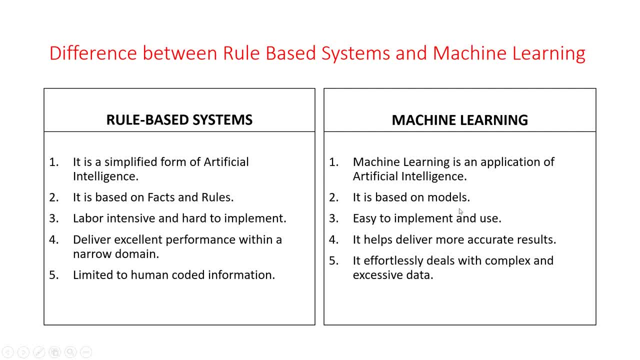 and rule. machine learning is based on the models. okay, there are different models are present in the machine learning model. it will have both the intensive and the hard to implement. it is easy to implement and use. deliver the excellent performance with the. 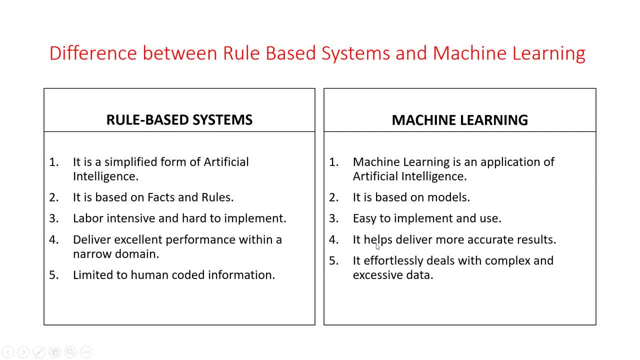 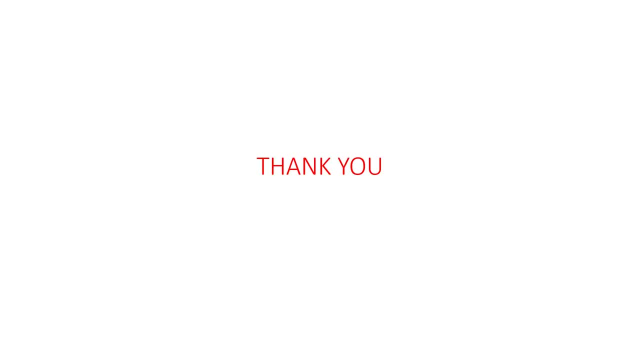 narrow domain, it helps to deliver the more accurate result. and, last point, is a limited to the human coded information and it effortlessly deals with the complex and extensive data. okay, so this is the difference between the rule-based system and the machine learning. so in the next video we are going to discuss about the types of rule-based system that.